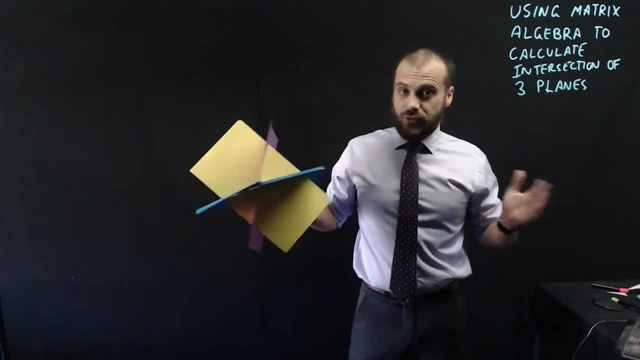 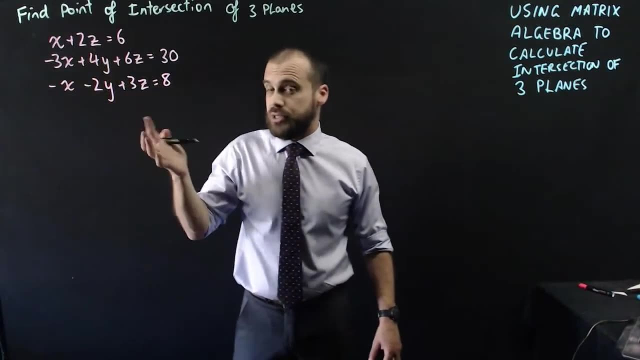 going to work, You'll need a different technique, So doing this is really straightforward. You've actually done it before, So we have three planes here Now. you'll notice straight away that this doesn't have three variables in it. It doesn't matter, It's just 0y in there. Okay, but these are. 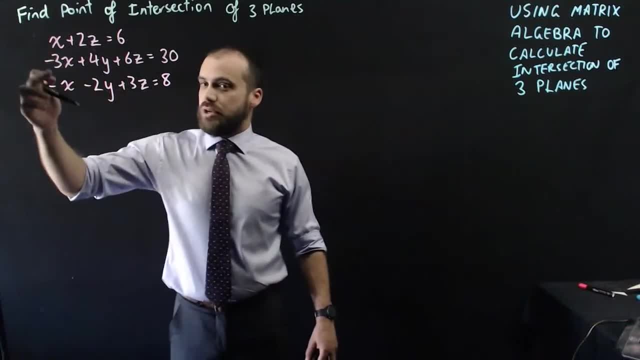 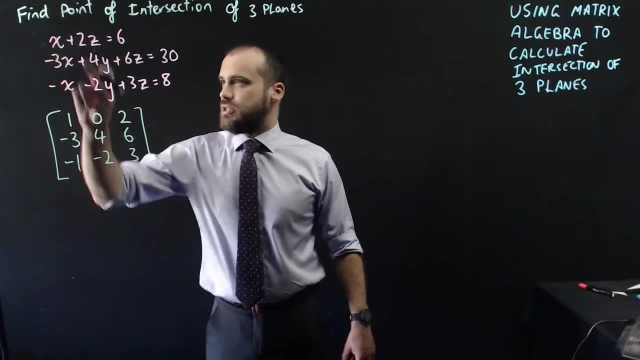 three planes. Now we can write these three equations into a matrix. So I've taken all of the coefficients and placed them in this matrix: 1x, 0y, 2z negative, 3,, 4, 6, negative. 1, negative. 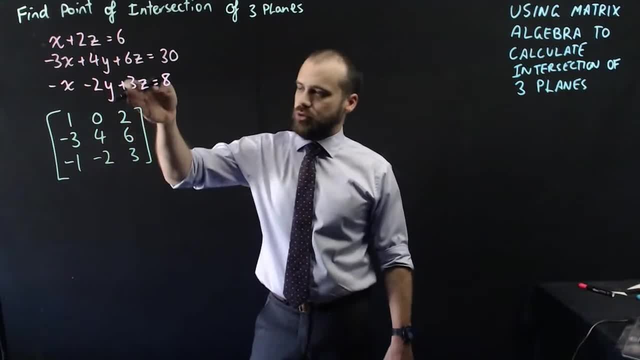 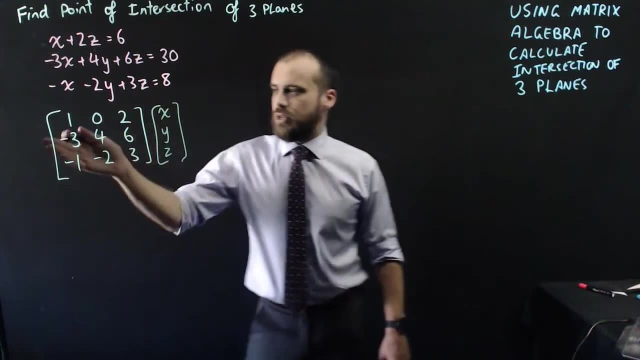 2, 3. Make sure that you put all your x's here, all of your y's here, all of your z's here, even if they're written in a different order. Okay, and there we put x, x, y and z there. Now, if we did matrix multiplication here, we'd end up spitting out. 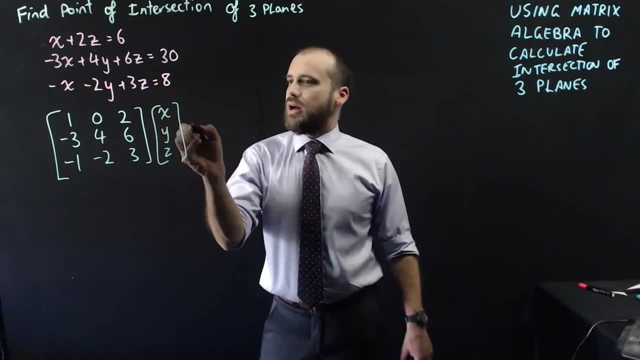 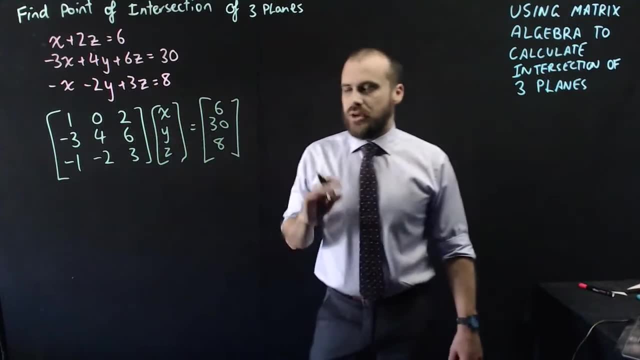 these equations right: 1 times x, 0 times y, 2 times z, And then that's going to be equal to the solutions here: 6,, 30, and 8.. All right now matrix algebra. you should remember your. 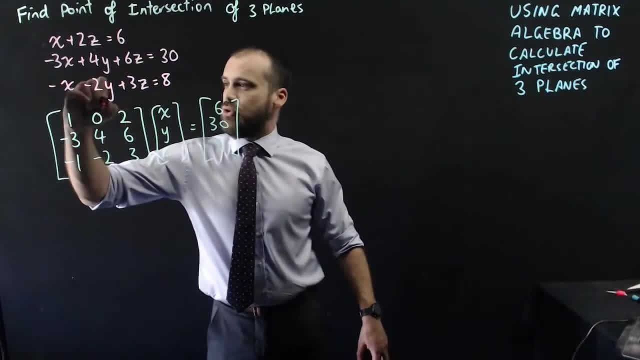 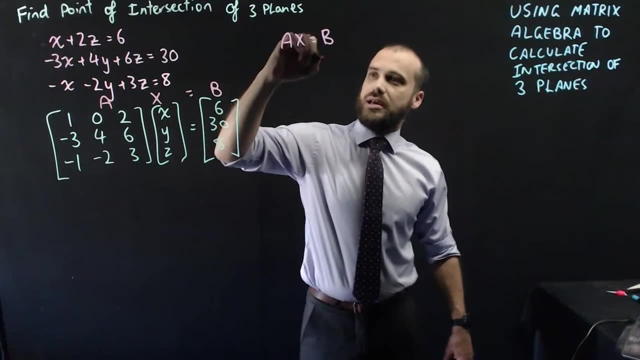 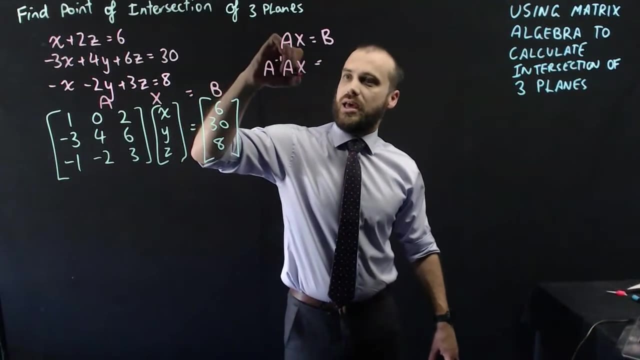 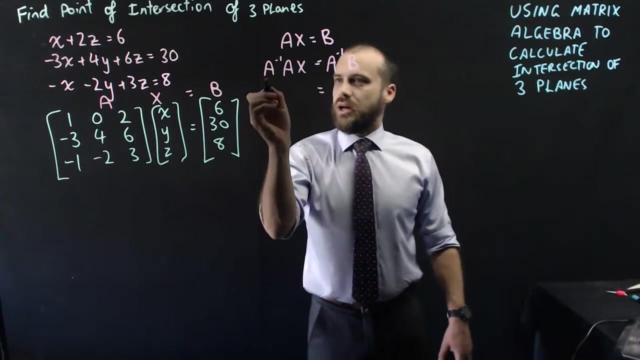 matrix algebra. This equation is of the form ax equals b, right? And you should remember that if x equals b, we can do something called pre-multiplication and say a to the negative 1ax equals a to the negative 1b. So we're taking the inverse of a and pre-multiplying it Now. 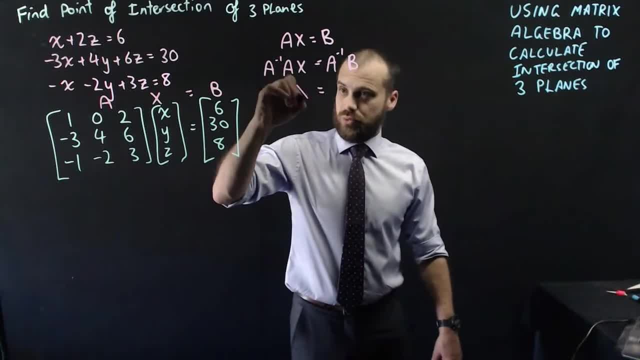 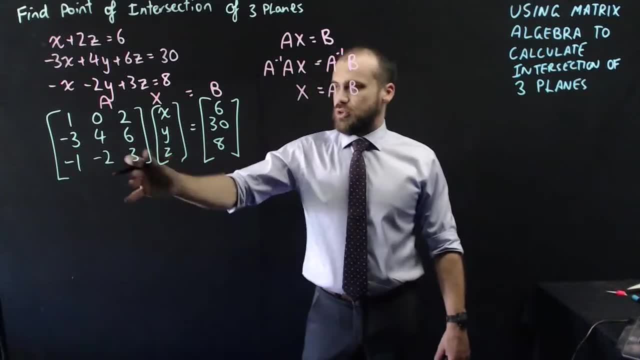 a to the negative 1 times a. that's the identity matrix, which just leaves us with x here and that's going to be this bit here, All right. so that means that to solve this, we rearrange it by bringing a to this side, but the inverse of a to the negative 1b. So we're going to do this. 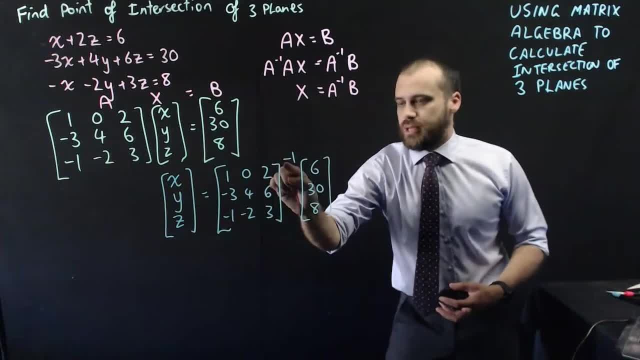 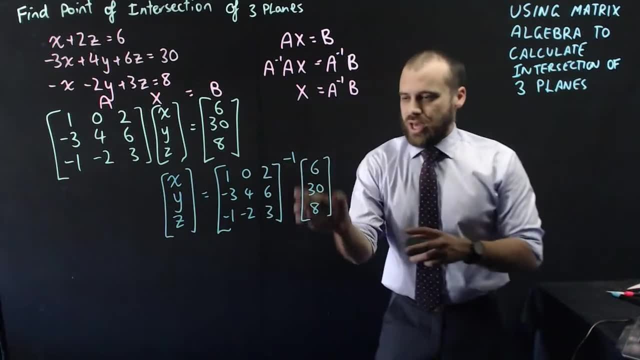 of that. So I've done that here, I've taken this, I've brought it over here, but as the inverse. Now you should be able to type that entire thing into your calculator, multiplied by that entire thing into your calculator, and we should get a 3 by 1 matrix.